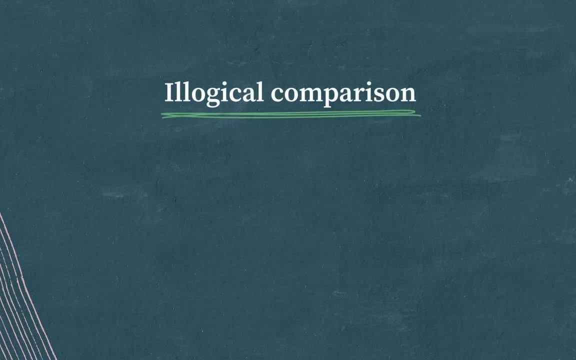 So an incorrect example, an example of illogical comparison would be: I prefer apples over people who love pears. So why is this incorrect? Because the sentence to people, not apples to pears, And a person is not picked in an orchard. It's not the. 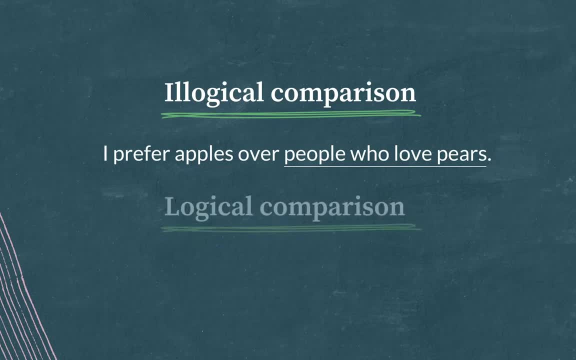 same thing. A person is not fruit. To fix this sentence, I need to compare apples to pears and change it to: I prefer apples over pears. You might need to add a word like that, or those, in order to correct an illogical comparison. Pierre's croissants are less tender. 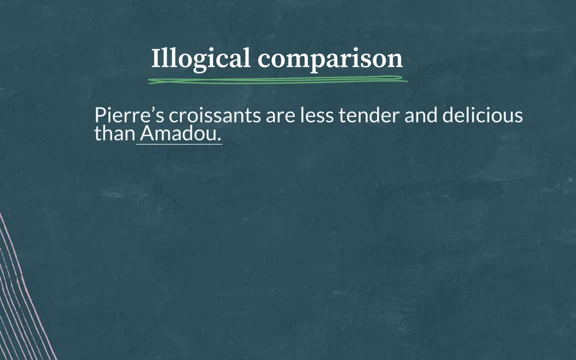 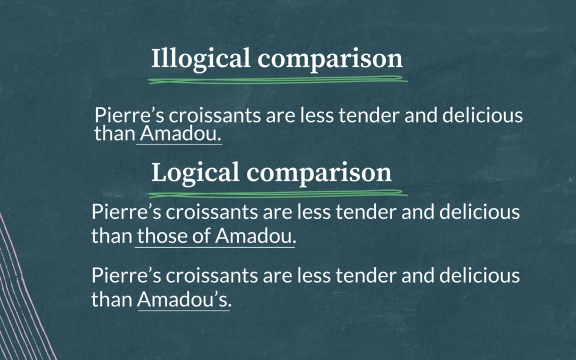 and delicious than amadou. This is an illogical comparison, because amadou is a person, not a pastry, So we want to compare his pastries to Pierre's. Pierre's croissants are less tender and delicious than those of amadou, Or Pierre's croissants are less tender and delicious than amadou's. 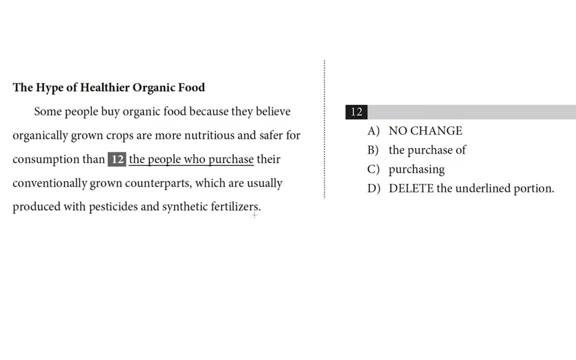 Let's go back to the question. Feel free to pause the video here if you want to take a crack at it yourself. Okay, let's do it together. I'm going to plug the options into the choices and see if the comparisons are logical. So people who buy organic food believe that they're 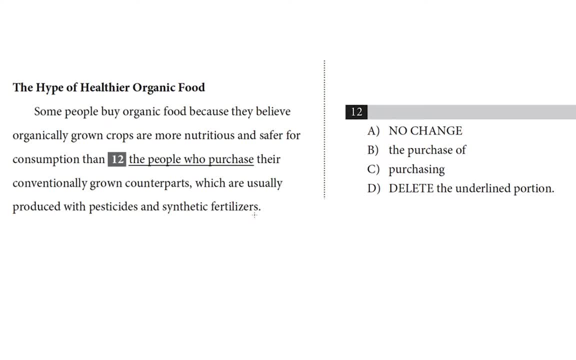 organically grown crops are more nutritious and safer for consumption than choice A, the people who purchase their conventionally grown counterparts. So organically grown crops are more nutritious than people. I don't think we're talking about eating people here, That's. 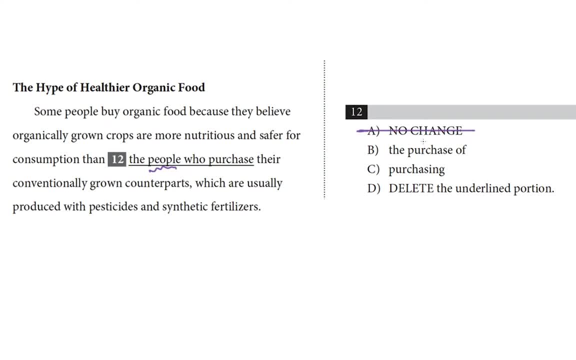 an illogical comparison. I'm going to cross off choice A. Choice B: organic crops are more nutritious and safer to eat than the purchase of their conventionally grown counterparts. Now we're comparing organic fruit and vegetables to the purchase, So I'm going to cross off choice C: the buying process of conventionally grown fruit and 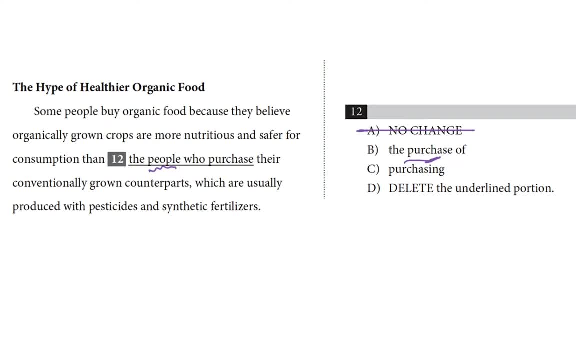 veg, And that's illogical. It's comparing fruit to the act of buying fruit. I'm going to cross off B. Choice C is purchasing and that's basically the same as choice B. Remember, when two choices on the SAT are functionally identical, that's a great way to know they're. 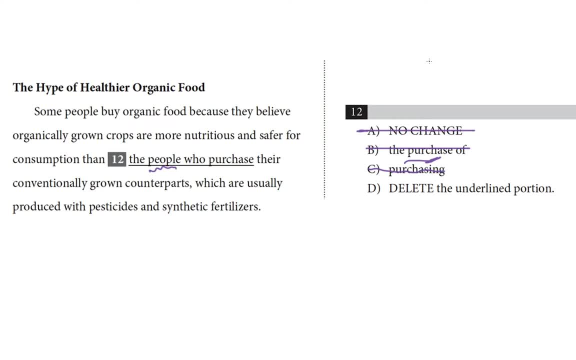 both incorrect. They can't both be right, which means they must both be wrong. So I've crossed it off. Toodaloo choice C. And that leaves choice D. Let's see what happens if we delete the underlined portion.